So the purple planet, for example, is a planet that goes right in front of the star and it's going to do a little bit of an eclipse on the star, so the brightness of the star that you get on Earth decreases during a certain period of time. 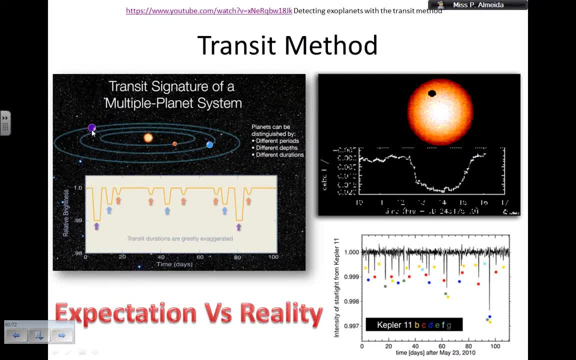 So that planet is pretty big comparing to the other planets. also because it's further away, it eclipses the star a little bit more, so this one is going to cover the star more, so the brightness decreases the most okay. 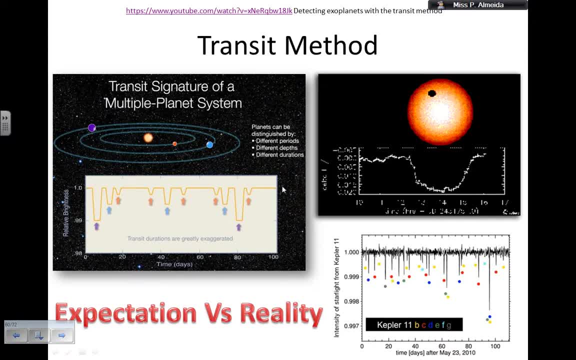 And I see this happening- exactly the same type of decrease in brightness over and over again. so this is something that is happening over and over again. possibly there is a planet around the star, so this is how the transit method works. Let's go on the blue planet. 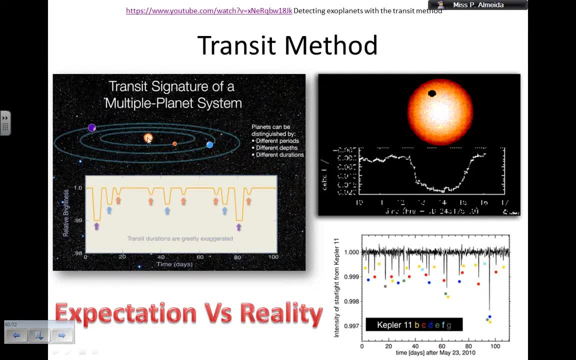 That one also a little bit bigger, but also further away from the star. so it makes more of an eclipse, and there is here the dip in the brightness which is always the same for the same planet. and then again it happens over and over again. and if it happens over and over, I think: okay, come on, I definitely have a body around that star, possibly a planet. so is it going to be an extrasolar planet? 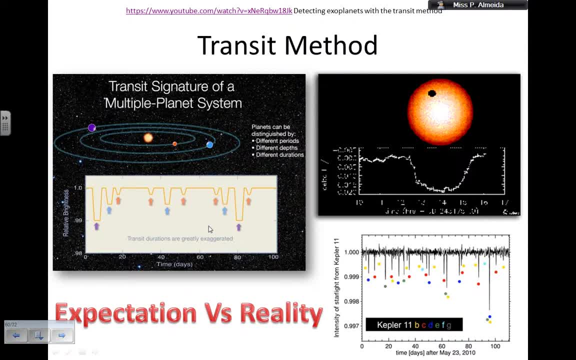 And you keep doing observations to confirm that there is an extrasolar planet. You can use other techniques. You can use other techniques, like radio velocity, for example, to confirm that it is an extrasolar planet. Finally, let's go on the orange one, this tiny one, closer to the star. 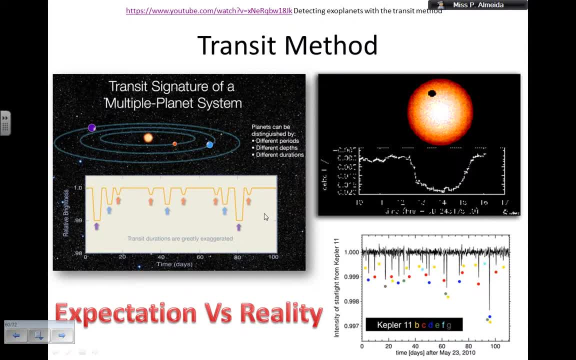 It makes a tinier bit okay because it doesn't cover as much as the star. and now let's look at all the lines together. The orange one is the closest one to the star. The repetition of the dip that I have in the brightness occurs more frequently because the planet is of course going to obscure the star more often. 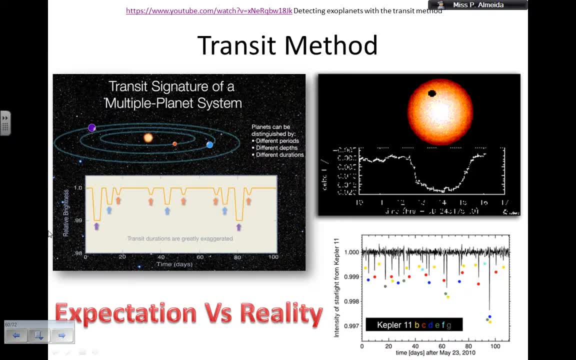 For example, the purple one. So this transit method is going to give me, just by looking at the light curves, information about how many planets I may have in there. okay, and I need to be careful. You need to say may. 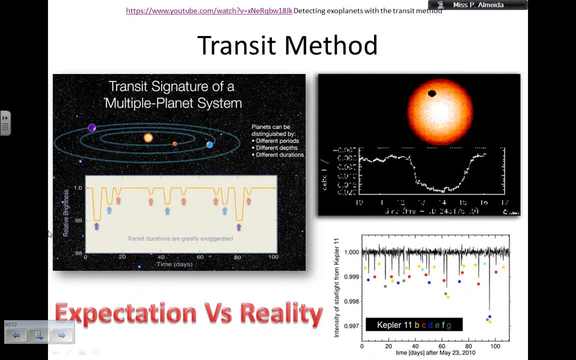 I mean, of course it can give you information about how many planets it has there. but we say may because you know it could be that there is a planet that is actually just the orbit is so oblique that you cannot even have it to cover the star. or it can be this: the covering of the star. 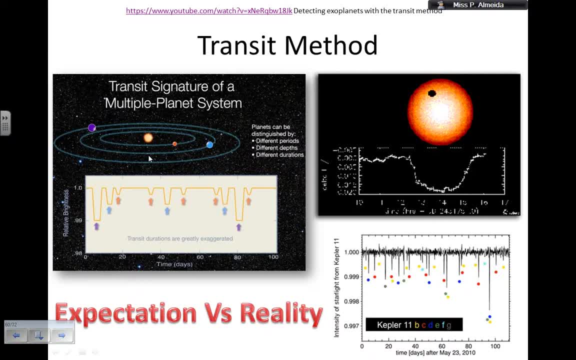 And you know what is this? Can this be the thing that covers the star? This is why I'm such a fan of the star. I mean, you know, the star can be confused with noise, which I'll go into in a second. 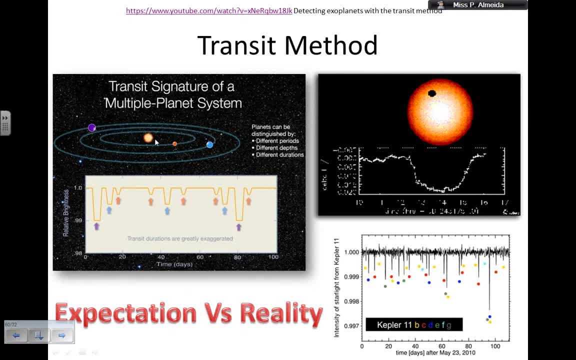 And then this one, the purple one. I mean possibly it's quite big, or it could be that it covers the star like much more. And look, the period of this orbit is not as large as the other ones. so you get a lot of information about the system. 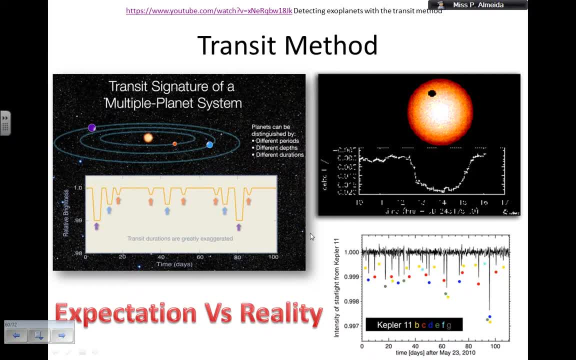 And it works really well with multi-planet systems, because you're going to have different dips. Again, this is an example of the Kepler-11 system, which was found using thermo-elemental mapping. So let's look at this, because it's quite big. 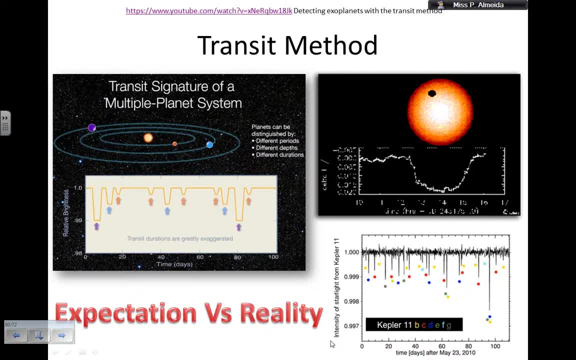 I mean, you know it's not going to cover the star, but it covers the star much more using- guess what? the kepler space telescope, which was sent to space just for look for planets. okay, using the transit methods. so this is the data, and different colors again correspond to different 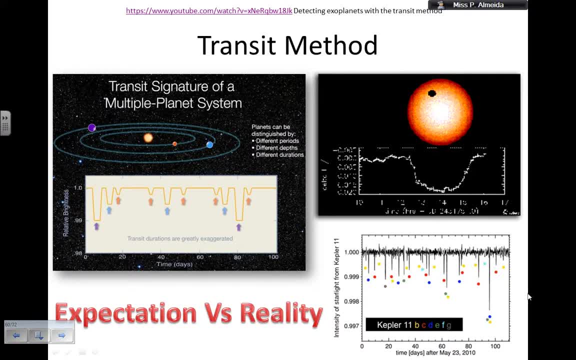 planets and you can see that according to the how much my brightness decrease, i can figure out that that is the signal, that is the pattern that my planet does. okay again. you also get information about the size of the planet, the mass, the orbital period, in terms of how close together these steps. 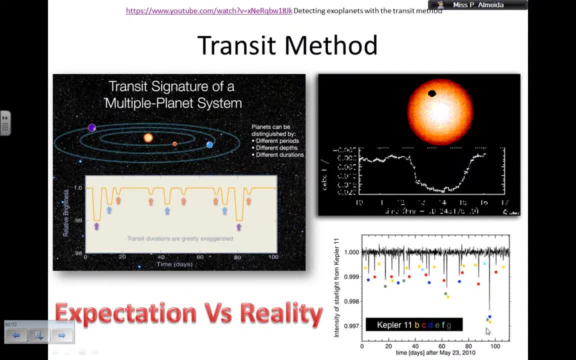 happen, and let's look at this example. sometimes three planets can be looking, uh, going around the star or in front of the star. so here here we go. at times you may have, um some not so frequency, frequent events where the brightness decreases much more. now, problem about this method is that 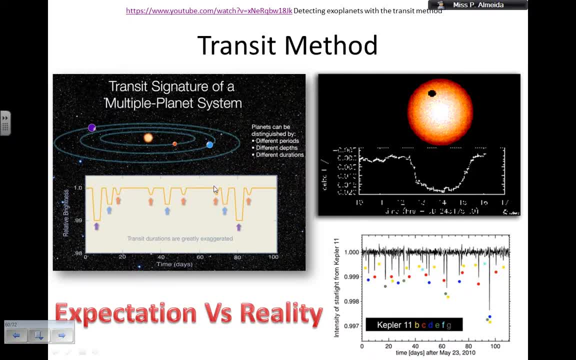 again, this is the expectation. really, nice curved lines or a straight lines, really, uh, and this is the reality. i mean, there is a lot of ups and downs, okay, and why. you know what? could this be a planet in here? could this be a planet? could that be a? 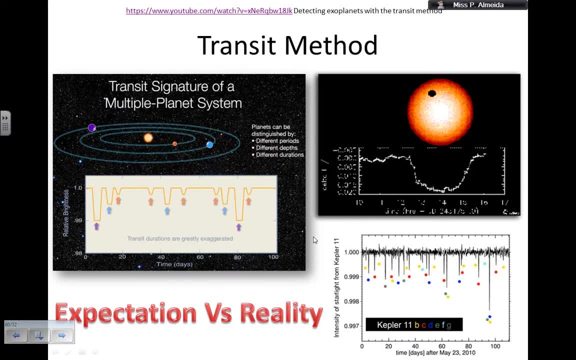 planet. so sometimes you don't know things for sure. okay, so the, of course, as any technique is not great, it's not perfect. i mean it's great actually, but it's not perfect, and sometimes is it really a planet in there. okay, so you can look at other techniques. all right, so i'll. 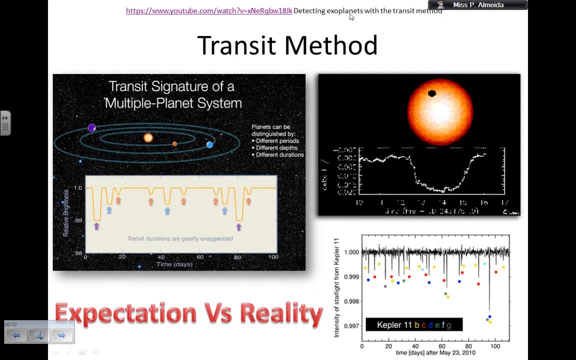 put the link of this video in the description. this is really just seeing. I don't know if this is even from the video, I don't think so, but it's really just seeing a planet going in front of the star, reducing its brightness and moving away from the star, and that's all that the video is. it's like you know. 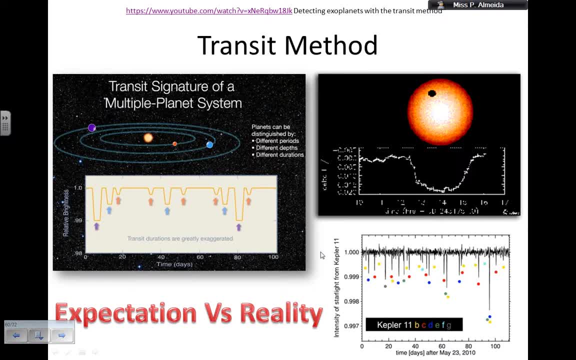 about 10 seconds, something like it, and you can also decrease the speed of the video if you want to see something that is very interesting. how fast, how steep this line is is going to give you an idea of the radius of the planet, which is going to be super important for something else that I'll tell you in a 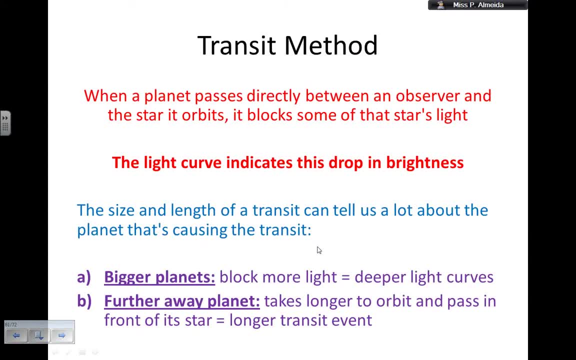 second. so transit method. when a planet passes directly between an observer and the star it orbits, it blocks some of the stars light. so the light curve indicates this by dropping in brightness. okay, the luminosity of the star is the same, is still emits the same amount of energy per second. however, the brightness that I 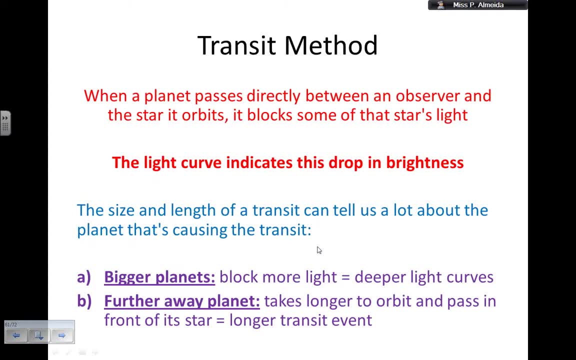 receive here on earth. changes, okay decreases, when the planet is blocking the light. the size and the length of a transit event can tell us a lot about the planets that is causing the transit. for example, bigger planets: they block more light, so the light curve is a little bit deeper. further away planets: they take longer to orbit. and 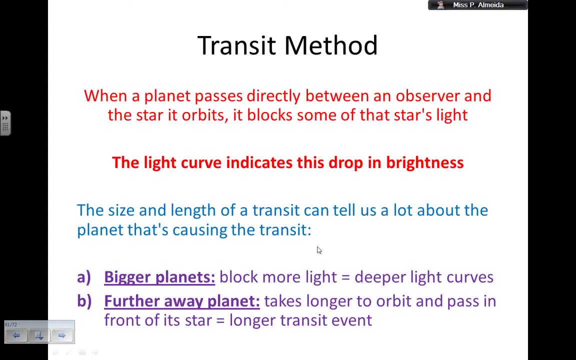 pass in front of the star, so the longer the transit events. okay, so you get a lot of information just by looking at the light curves. and again, this method is biased towards a certain type of planets. think about it: bigger planets. if the planet is bigger, it blocks more of the light. I do not confuse the deep in the 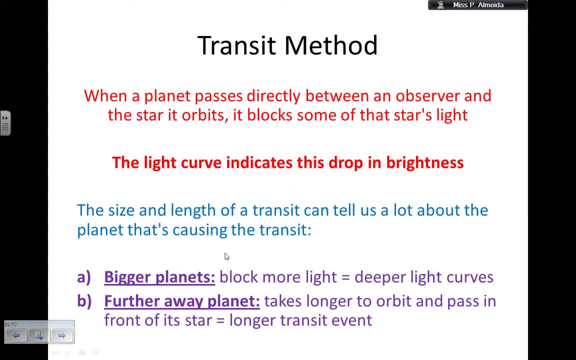 brightness, weeds, noise, okay. and obviously planets. they are close to the stars because they are going to pass around the star more often, so I can more easily find out that there is a planet. I don't have to wait ten years until the next transit event and say, oh yeah, that's going to be a planet, okay, so the 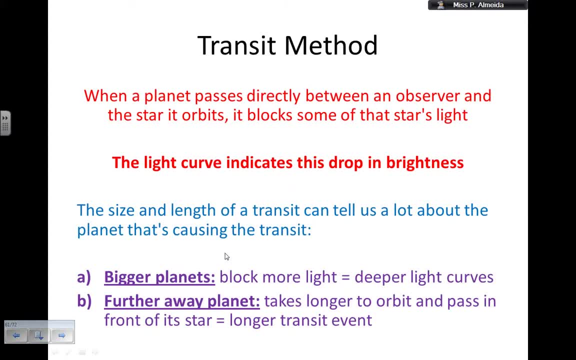 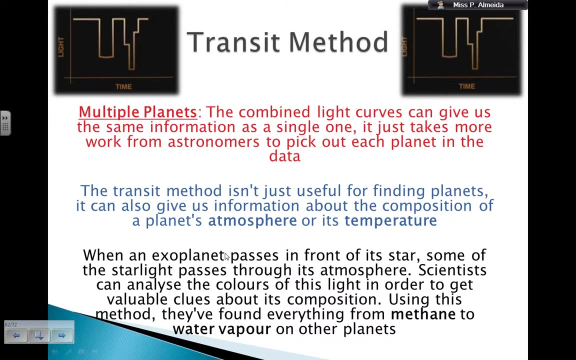 transit method, just like the radial or doppler velocity method. they are biased towards hot jupiters, which are planets. they are quite massive and they are traveling very close or orbiting very close to the star. okay, so multiple planets is actually quite good for multiple planets and 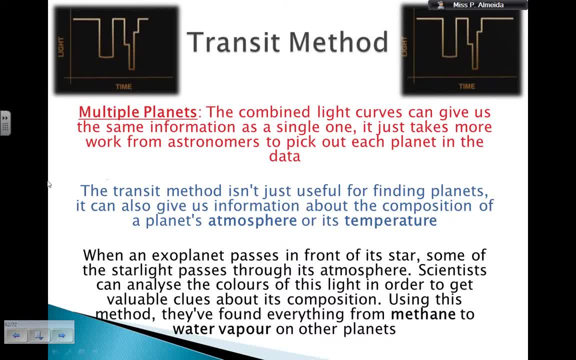 again another example in here: okay, the combined light curves can give us the same information as a single one, so it just takes more time for us to pick up and pick out which planets is in the data, which planet is contributing on how much on that deep in the light curve. okay, and the? 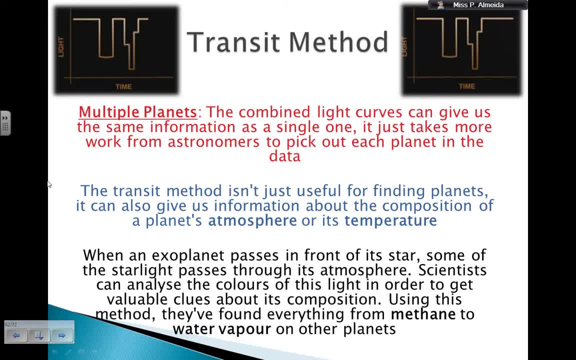 transit method isn't just useful for finding planets. it can also give us information about the composition of the planet's atmosphere or its temperature. okay, and this is again when i combine data, because i have a transit event and i can easily get the radius from the light curve. okay, and i can easily get the radius from the light curve. okay, and i can. 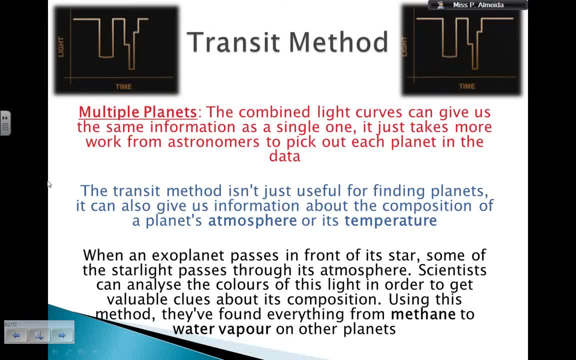 easily get the radius from the light curve. okay, and i can easily get the radius from the light curve, or from what is the steepness of my curve, when i get the right the transit event then, and i know how massive the planet can be by looking at the deep. then i can look at the density, because mass 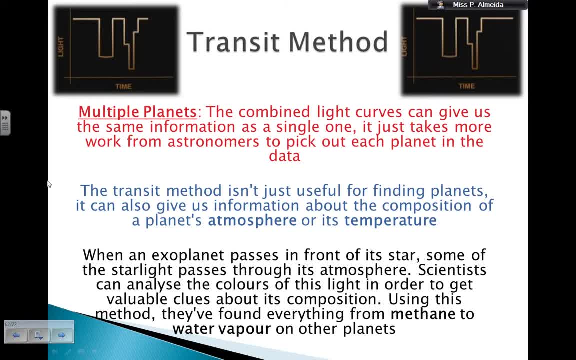 is density? is mass over volume right? so i can have an idea of the density of the planet, i can figure out if he's a rocky planet or a gaseous planet, and then, just by looking at the transit event, i can also take up or pick up data about the atmosphere of the planets. 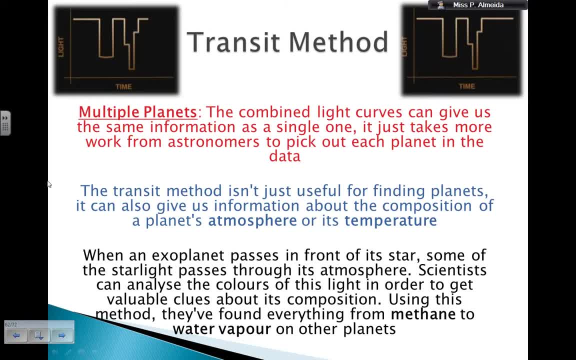 okay, and there it is. when an extra planet passes in front of its star, some of the star lights passes through its atmosphere, so the scientists can analyze the colors of this light in order to get valuable clues about its composition, the composition of the atmosphere, using this method. 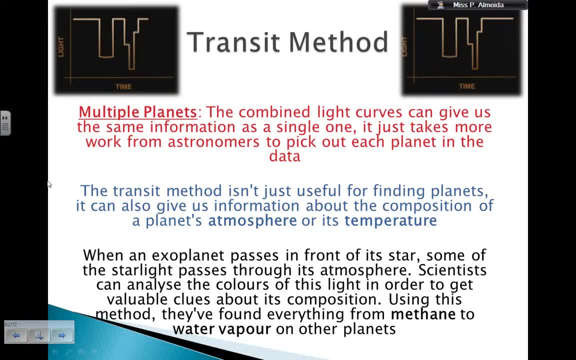 they found everything from methane to water vapor on other planets. and why is this important? well, if a planet has methane and water vapor in their atmospheres, uh, they have an atmosphere that is at least a little bit similar to ours, so maybe they can harbor life. maybe they can have this amount of greenhouse, if uh effect or 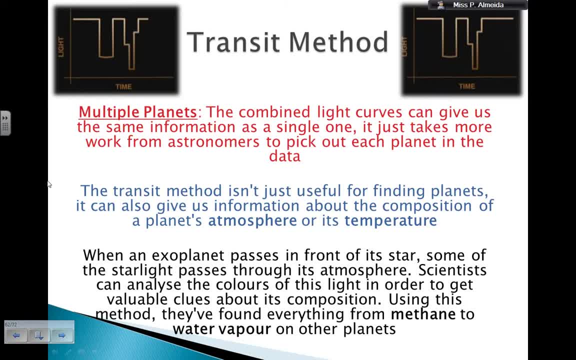 yeah, that is enough to keep the planet warm, even if it is not facing the star at that particular time. okay, the greenhouse effect is something that is actually. without it, we wouldn't have life on earth. it's just that if it's an extreme greenhouse effect, then it's going to cause global warming. 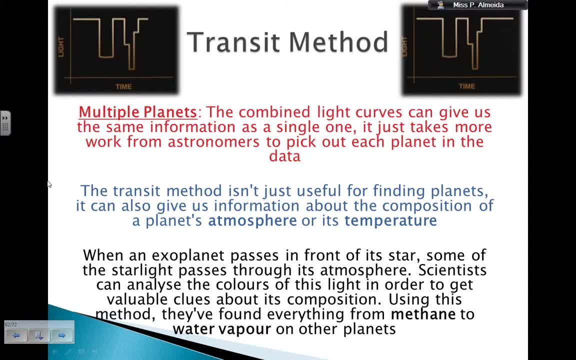 okay, but this can be in another video. so, uh, and this is very important and let's think about it. i mean, we have so many techniques to find out planets. they are so successful. why did we send a telescope to space for this? well, if we're looking for planets that could be like our own,